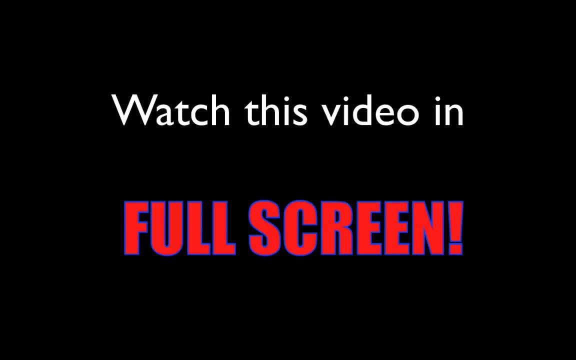 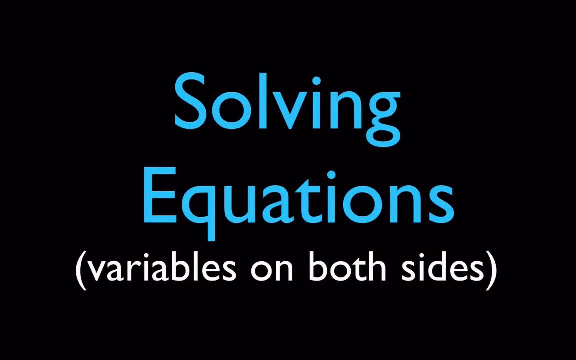 Okay, everybody, what we're doing today is we're going to take a step back, And this is something you guys really enjoy doing, which is solving equations. You're pretty good at that, So this is nice to get away from graphing for a little bit. And the reason 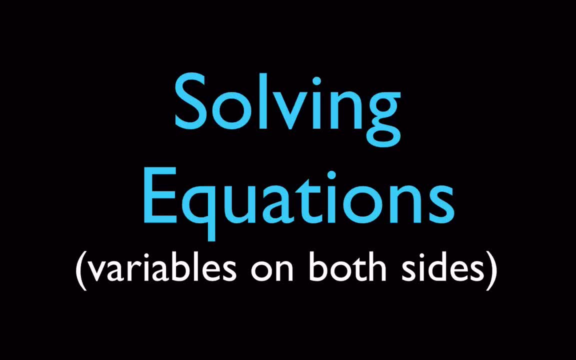 we're going ahead and going back to solving equations is because we're about to start solving systems of equations, And by that I mean we're going to be finding the place where two lines cross each other. But you don't have to do that using graphing You. 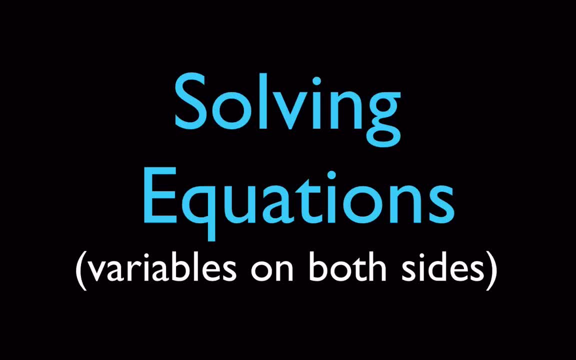 can do that using algebra, And it's actually much, much better to use algebra to do it because of the inaccuracy of graphing. What that means is we're going to be solving the only type of equations we haven't solved yet, which are when you have an X or any letter. 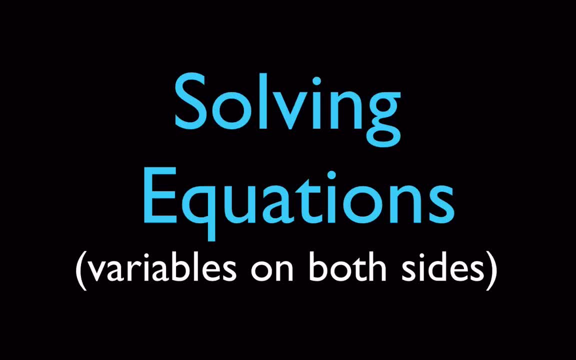 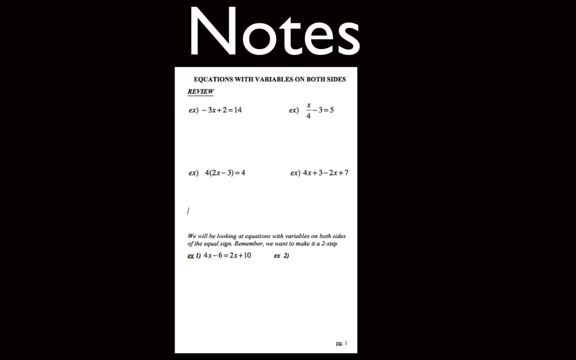 but in this case X on both sides of the equal sign. Before we do that, though, I want to start doing this now. It's pointing out the notes you guys should have out right now. Okay, so this is. you have two pages of notes. This is the notes you should have out in front. 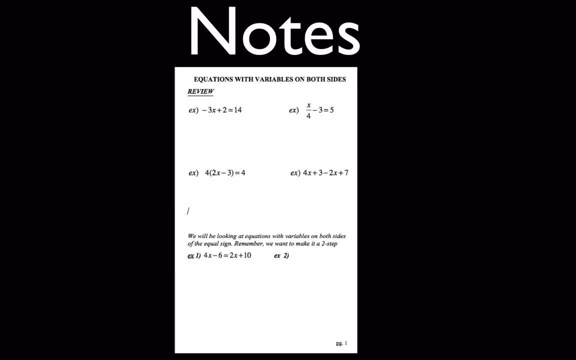 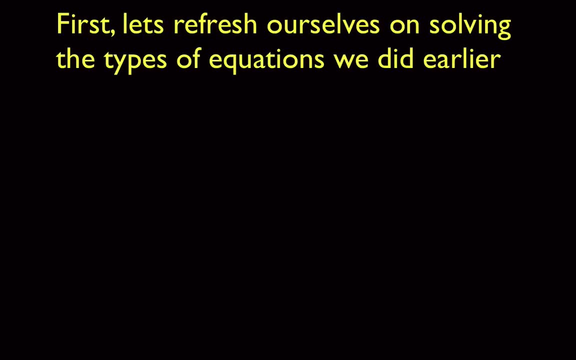 of you right this second. All right, before we go ahead and jump into something new, I want to make sure you guys remember how to do the older stuff. So we're going to go ahead and go back over one-step equations, two-step equations and then multi-step equations, three or four-step equations, Making. 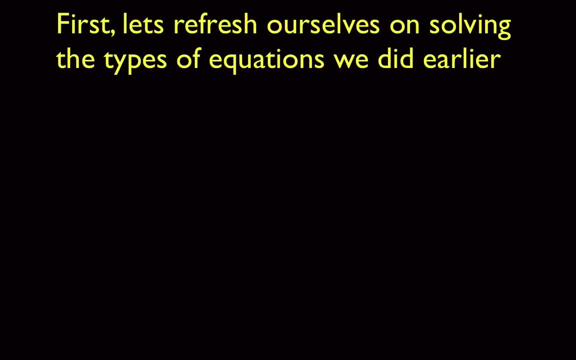 sure that you guys remember how to do all that, because even with variables on both sides, you also have to incorporate combining terms and distributive property And, just like everything else, you're trying to get the problem to a two-step equation. So here's the first example. 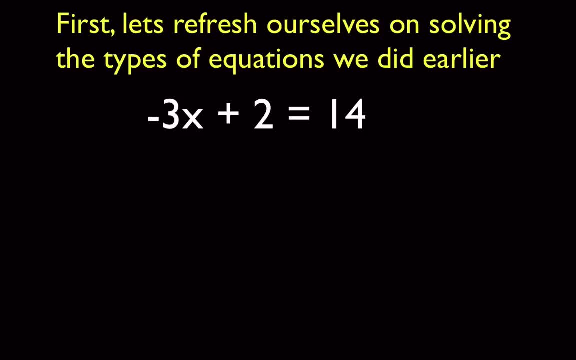 This one's already on your page. What you could do is you have two choices: You can go ahead and watch the video, and we'll go ahead and go over the steps if you don't remember how to do it, Or you could pause the video and then we'll go quickly through the steps after that and make sure. 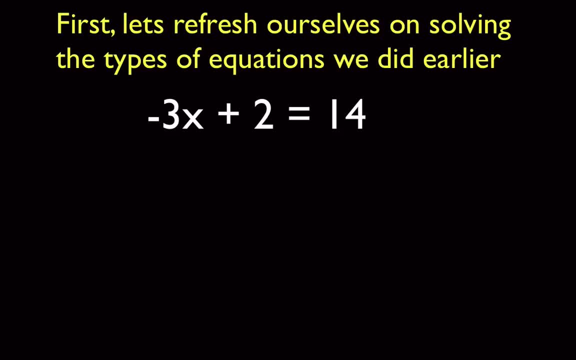 you have everything correct. So if you'd like to pause the video and try to do the whole problem on your own, go ahead and do that right now. All right, so what we're going to do is first, if you remember, we drew a line, Okay, and 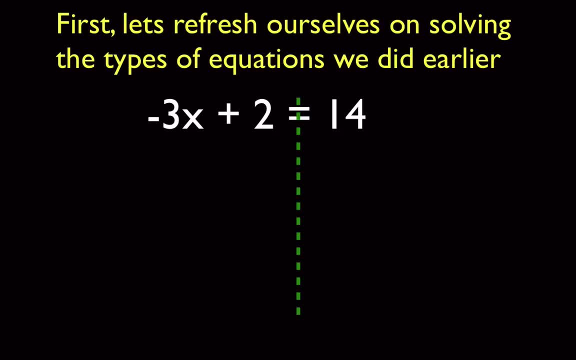 that was a step to keep us organized and keep everything straight up and down. Then we're going to do the opposite of what we did. So we're going to do the opposite of what we did. whatever is being added or subtracted to the x, So it's the number on the right. 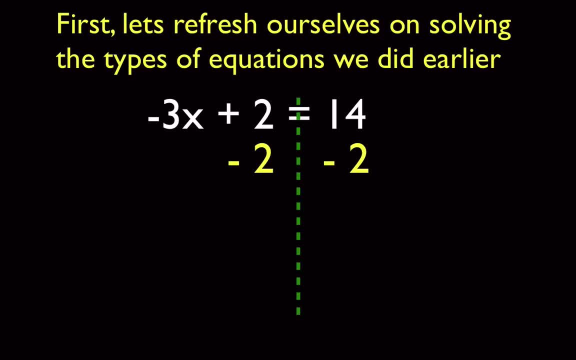 side. They can be rearranged, so the number is the number that's not attached to x. So I'm going to subtract 2 from both sides. that cancels out on the left side and leaves me with negative 3 x On the right side. 14 minus 2 is 12.. 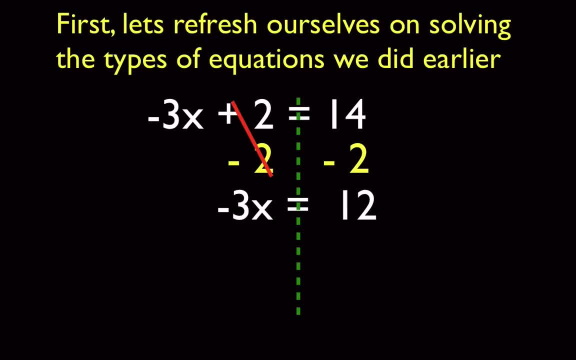 The next step from here is to get rid of that negative 3.. That's negative 3 times x. so we do the opposite, which is dividing by negative 3.. Negative 3 divided by negative 3 cancels out, and twelve divided by negative three is negative four. and that's it, you're done. 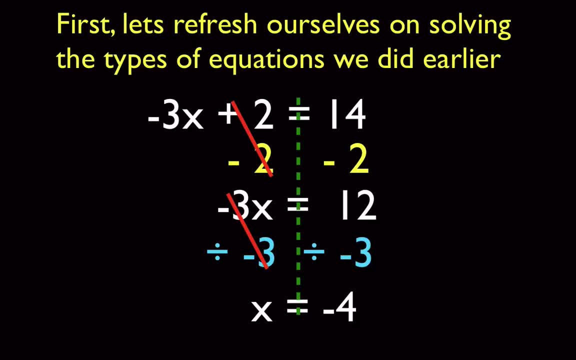 okay, so that's a two-step equation. the reason is: remember, you have two steps, step one. step one is right here. step two is right here. that's why it's called a two-step equation. okay, so we're going to do the other kind of two-step equation now. 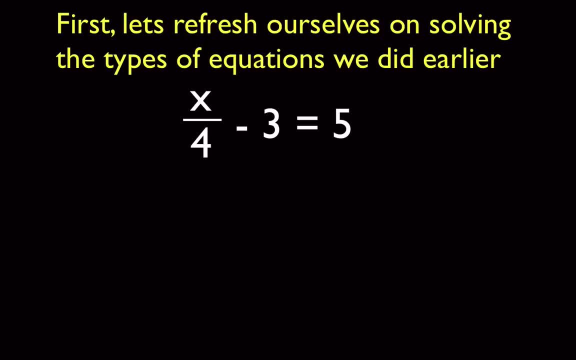 which is where you have division problem at the bottom. so instead of four times x, this is x divided by four, and remember there's a trick to this one, so be careful when you do this problem. so pause it if you'd like to do it all on your own. 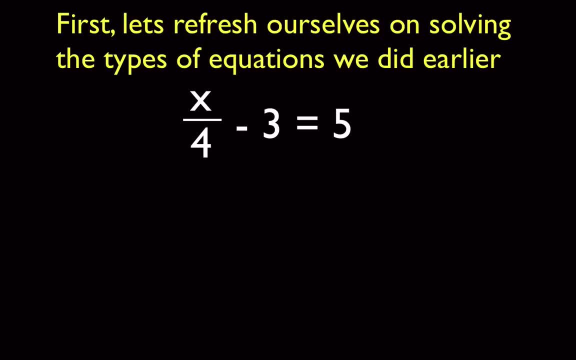 or just go ahead and let the video roll, if you want to go ahead and watch how to do it. alright, just like before, we're going to draw our line right away. we're going to do the opposite of subtraction three, which is to add three to both sides. 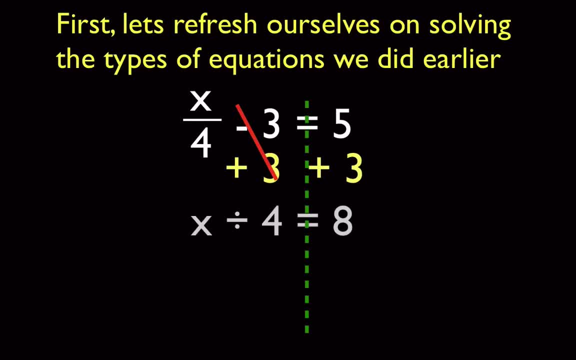 now my recommendation to you remember, is to go ahead and rewrite x over four as x divided by four, to help you remember that the opposite is not going to be division this time, it's going to be multiplication this time. this time now, we perform multiplication on both sides. 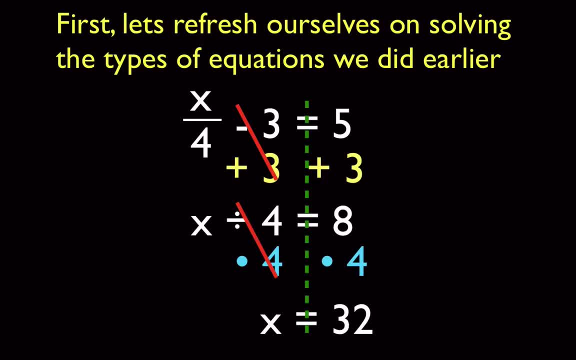 and we're going to get x equals thirty two. so if you did this problem incorrectly, you probably end up with x equals two, which is where you go ahead and you do this right here, where you have x over four equals eight, from right there, and then what you do is you go: oh okay, i'm gonna make these even so, i'm gonna go over. 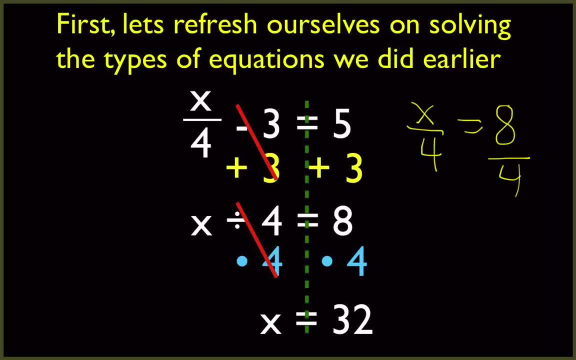 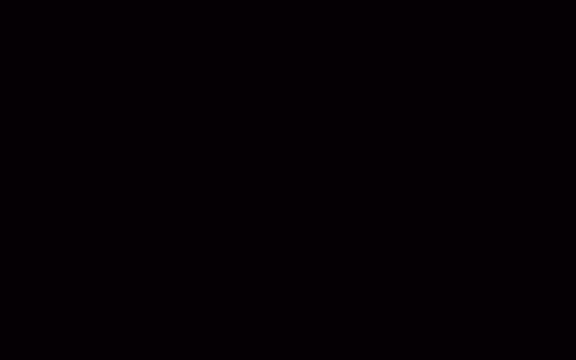 four, and it's a very common mistake to make, whereas when you have the division like we put right there, you do the opposite of division, which is multiplication. okay, now we're going to transition into three step equations. remember that that four on the outside is very important, and what we did in here is circled. 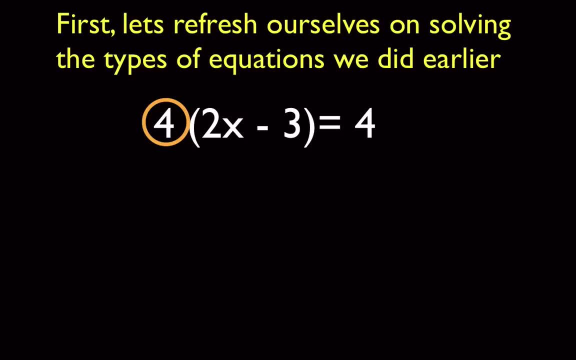 it. so go ahead and hit pause if you want to try to do the problem all on your own. if not, play the video and you can watch what happens, all right. so here we go. so i'm gonna take that number on the outside and we're going to multiply it by both of 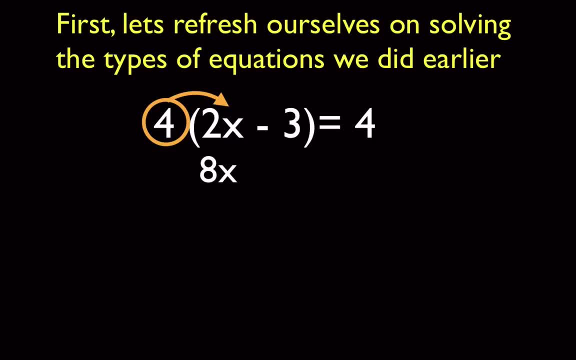 the numbers on the inside: four times two- x is eight x- and four times negative- three is negative twelve. okay, we're gonna bring down our equal sign and our four and now look what we have. we have a two step equation. very important to remember that every single time we're solving an equation, we're always trying to keep the 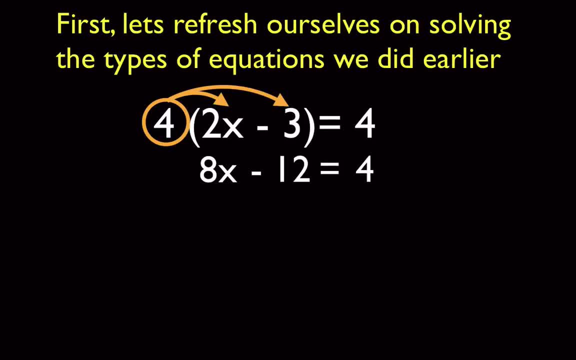 trying to get to a comfortable two-step equation, then we know what to do. so now we draw our line, do the opposite of subtracting 12, which is adding 12. that's gonna leave me with 8x equals 16. now it's 8 times X. so we do the opposite of. 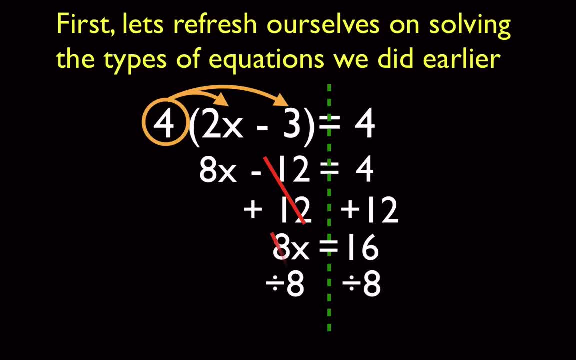 that, which is division, and we end up with X equals 2. okay, so, again, this is a what's known as a three-step equation, because this time we have our first step, our second step and our third step. a lot of times, though, they just call that a. 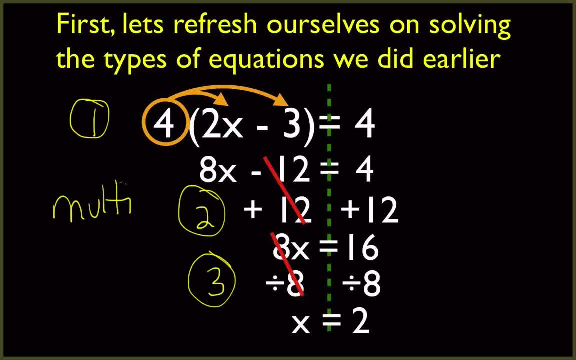 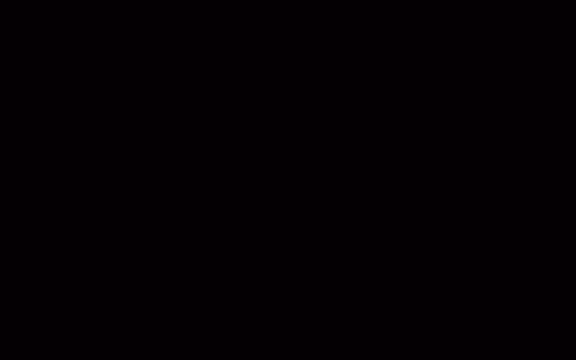 multi, anything more than two. they call a multi-step, and the big thing to remember is: you want to get to where you have just two steps left. okay, the last example before we move on. we have a multi-step equation here that consists of combining like terms. so go ahead and 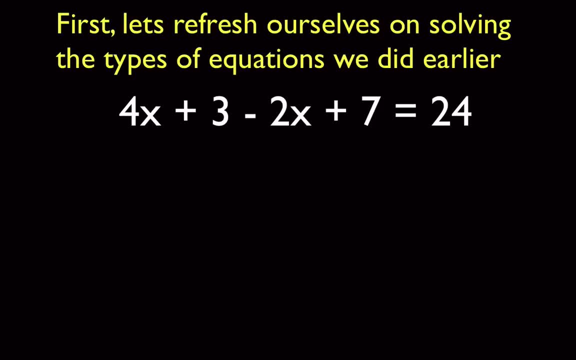 pause the video, hit play when you're ready. or if you want to just watch it, just go ahead and watch it. all right, starting off here, we're gonna combine like terms. the way we did combining like terms in class was went ahead and put a symbol around them. it's not the only way to do it, that's just the way I showed. 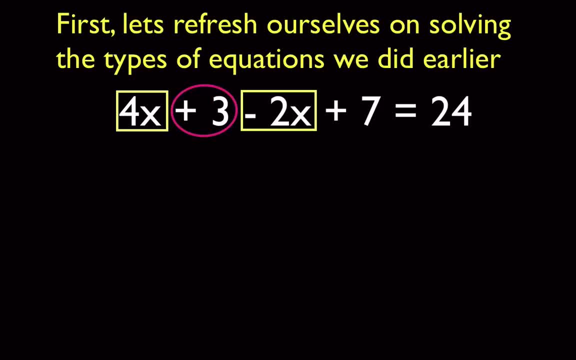 you guys in class. so we're gonna go ahead and group those first and I'm grouping things that are alike. now that I have that, I'm gonna combine like terms, and a lot of people have trouble with it like this, so what you could do is go. 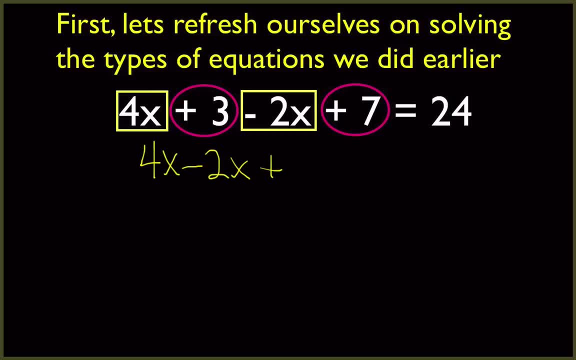 ahead and write it as 4x minus 2x plus 3 plus 7, and all I did there was I rearranged the like terms to be next to each other. so now I can just do that and I can just do that, and that's two separate, simple problems. so what I end? 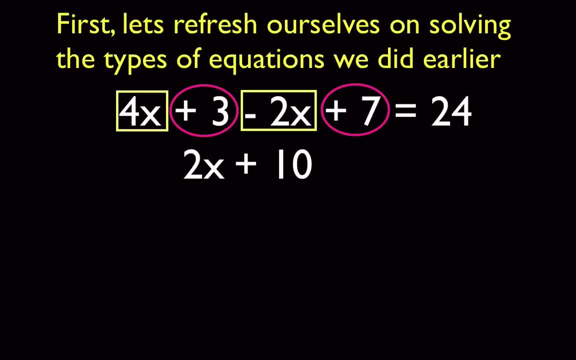 up with this: 2x, 4x minus 2x, and 3 plus 7 is 10. bring down the 24. now, what do we have? well, a two step equation. so at this point, we're just gonna follow the steps. we know. we're gonna go ahead and do that right now. 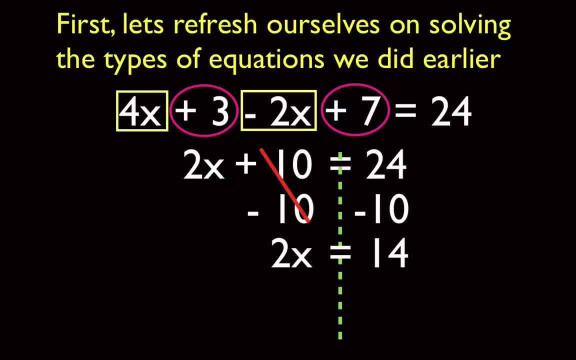 and subtract 10 from both sides and then divide by 2, and that's it. the problem is solved. what you're gonna find, luckily for you guys, just like you did on the multi-step equations- is that you usually don't end up with those division two-step equation problems, because it's very difficult. you have to add fractions. 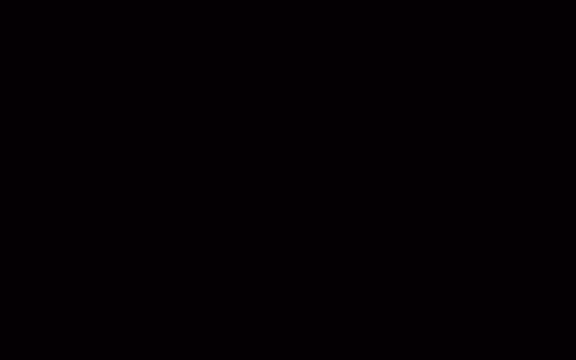 and stuff like that. okay, so what we want to notice here is that what every single one of those examples had in common was that they always had the variables that were on the same side, meaning all the X's were on the left side, and that's important, because when you do that, you don't have to do any moving of the X's. 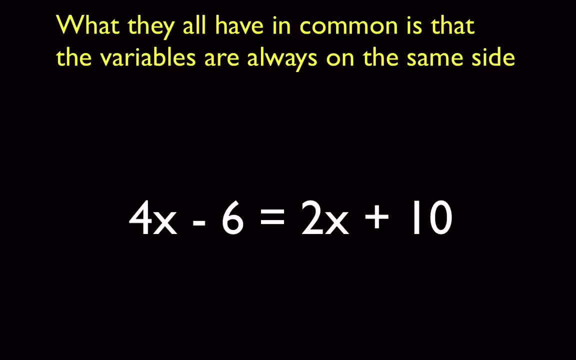 all you're doing is combining and adding them up. so here's an example of a problem that's a little bit different. what you'll notice is a. The variable is on both sides of the equal sign. So if I draw a line in here, I have x's on the left side and I have x's on the right side. 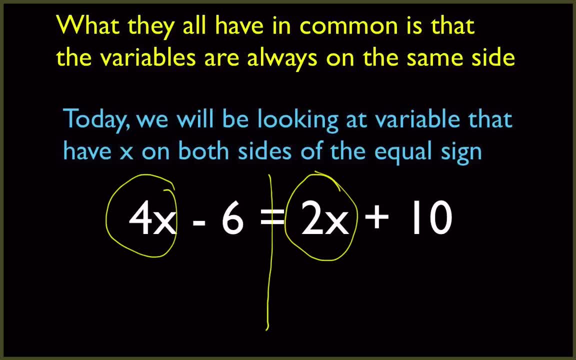 A very, very, very common mistake for people to do on these is to combine like terms. You can only combine like terms when they're on the same side of the equal sign. Be very careful about that. If they're on opposite sides, like this, you have to do just like you would do with the numbers. 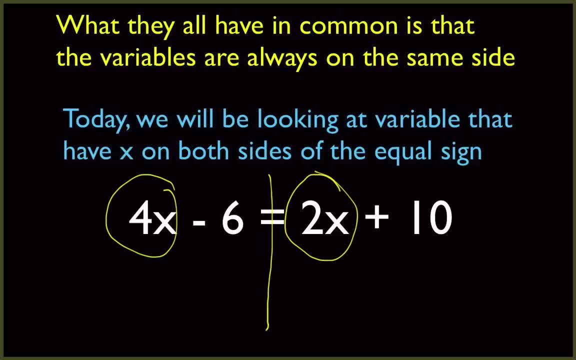 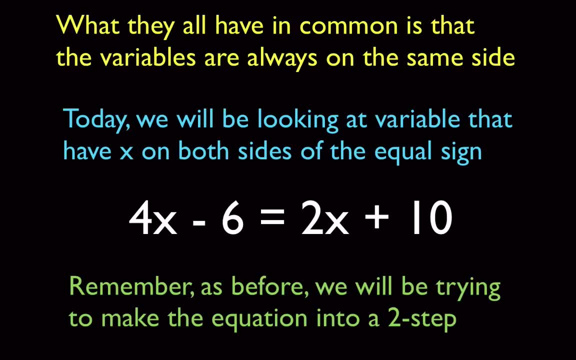 and you add one of them or subtract one of them to cancel out. So what we're going to do is we're trying to make this look like a two-step equation. So when I look at this I'm thinking, hey, that 2x on the right side shouldn't be there. 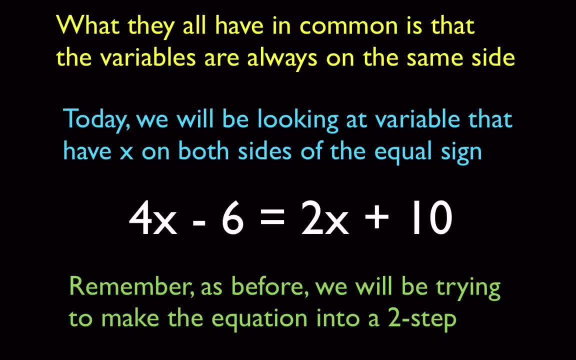 or at least the 4x shouldn't be there, But one of those x's needs to be gone for it to be a two-step equation And, like I said before, what we want to focus on is how is this different than a two-step equation. 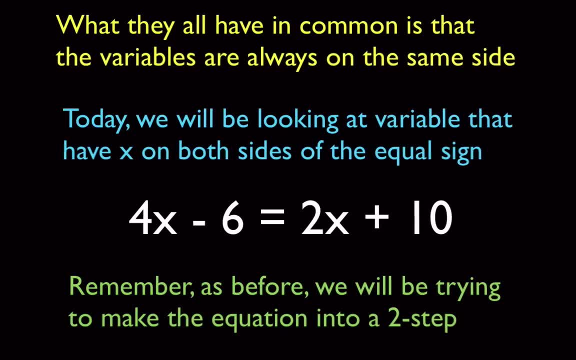 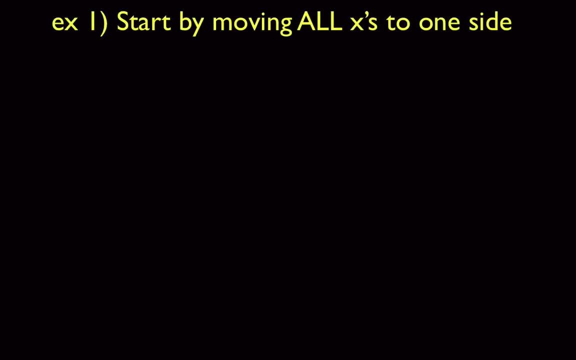 and what can I do to make it look like a two-step equation? Okay, so, first thing, we're going to start always by moving all x's to one side And you can see, on the right side we have a two-step equation. 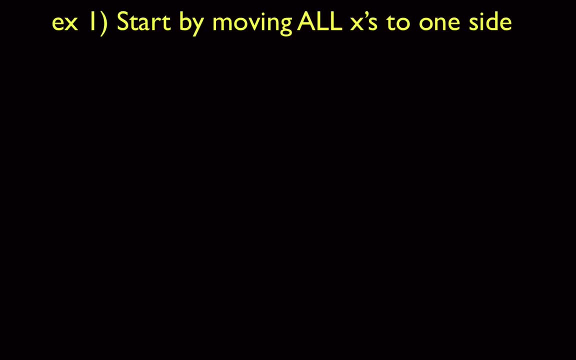 And you can see on your notes that you already have the first problem on there. Okay, so 4x minus 6 equals 2x plus 10.. Technically, this problem can be done a ton of different ways. You could go ahead and subtract 4x from both sides. 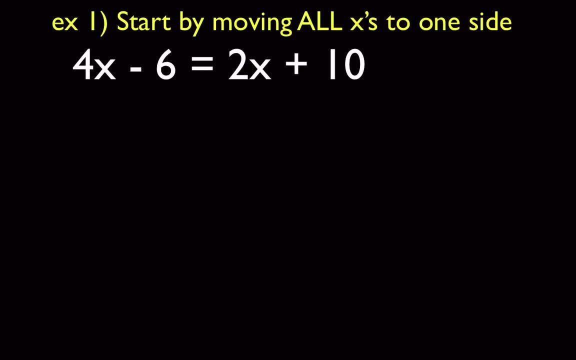 or you could go ahead and subtract 2x from both sides, But the key is you need to get rid of either this one or this one. My rule of thumb is: because I don't like dealing with negatives- my rule of thumb is to get rid of either this one or this one. 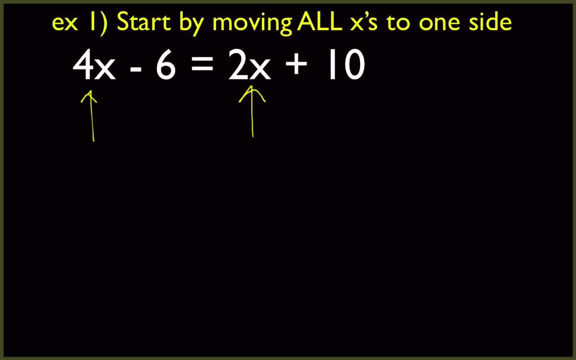 My rule of thumb is to always get rid of the lower of the two, the lower number. So in this case you could see the lower number is going to be 2x. But sometimes you've got to be careful because if it's something like negative 10 and 4,. 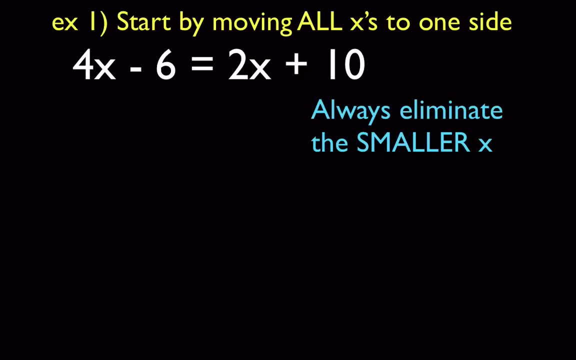 a lot of people will think: oh, 4 is lower, But it's not Think about. on the number line, Negative is definitely smaller than a positive number, So you always want the smaller number, the number that's either lower in the case of 4 and 2. 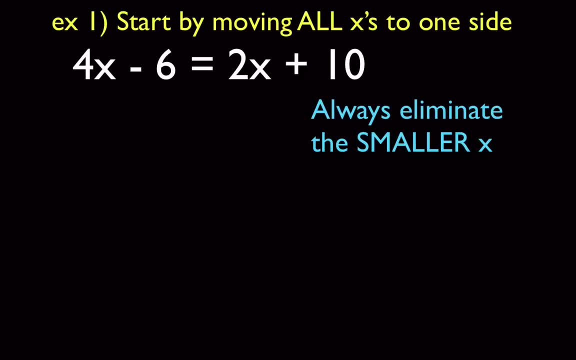 or if it's negative, it's definitely lower than a positive number. And what this does for you is all it does really- is it gives you a positive x to divide by, So you don't have to worry about negatives as much. So what we're going to do is we're going to add 2x to both sides. 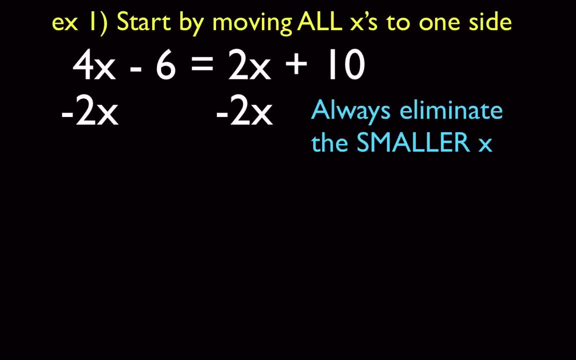 And the reason I'm doing that is because 2x is smaller. So think similarly to how we solve a two-step equation. After I do that, I'm going to end up with 2x on the left side, because 4 minus 2 is 2.. 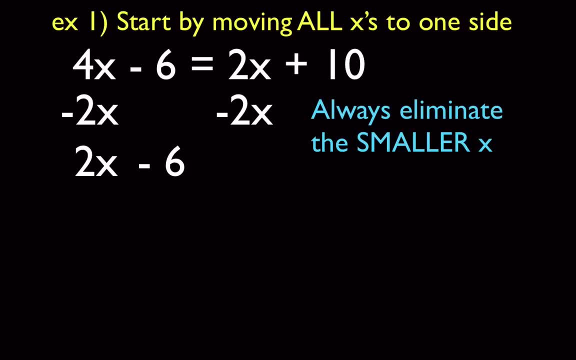 I'm going to end up with negative 6, because I haven't added anything to that yet. Those are going to cancel And that positive 10 is just going to come down. What do I have now? I have a two-step equation. 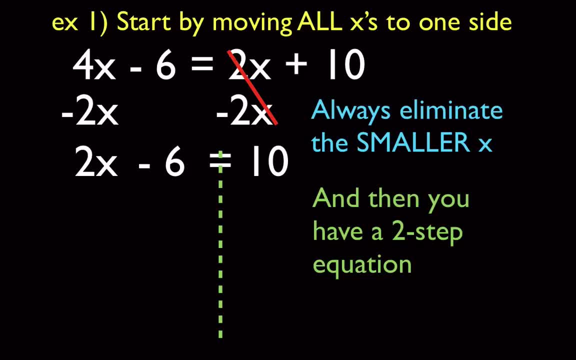 So now what we're going to do is we're going to solve it just like we normally solve two-step equations, So that first step is still just a three-step equation. That first step is to go ahead and get rid of the lower of the two x's. 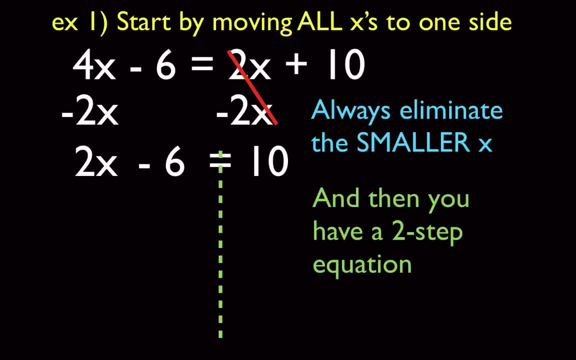 And the reason I want you to think about that is again. look at the problem originally And ask yourself: how is this different than a two-step equation? It has an x or x. Some people will always get rid of the x on the right side. 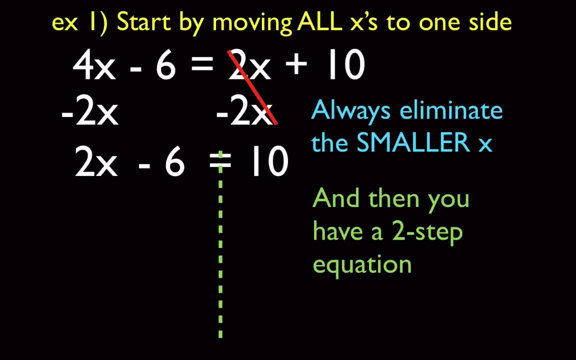 because they want it to look like a normal two-step equation. You can also do that. My rule of thumb, though, like I said, always get rid of the smaller one. Now we're going to add 6 to both sides, which is going to give us 2x equals 16,. 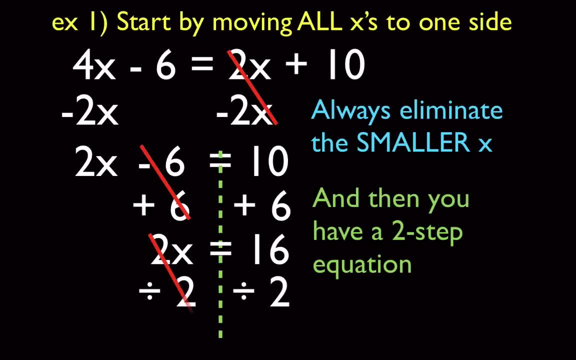 and then divide by 2 on both sides, which is going to give us x equals 8.. So make sure you fill this all the way out in your notes And, as you can see, it's just basically a three-step equation. First step: get rid of the extra x on the other side. 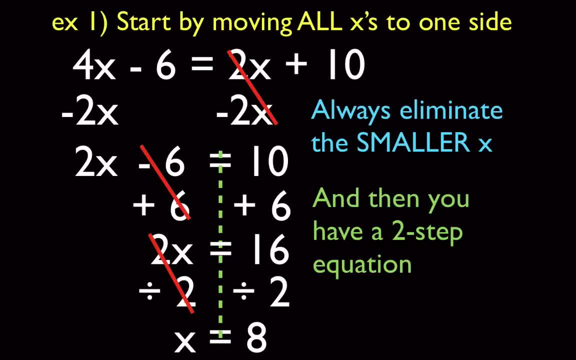 and go from there. I really want you to be careful not to combine like terms here. Remember that that equal sign means you can only do something on one, You can only combine and organize. You can only organize on one side of it. Okay, now we're on to the second example. 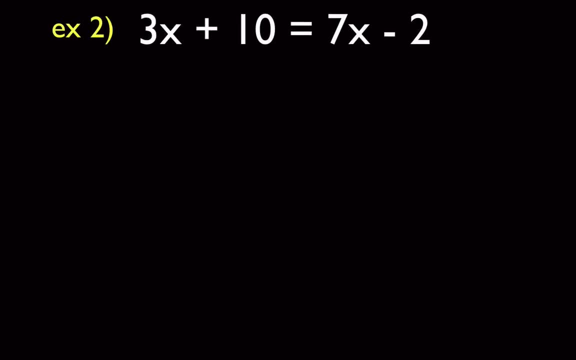 As you can see, it's blank, so you're going to have to write the problem down where it says ex2.. So I'll give you a sec to copy that problem down And we are going to go ahead and go through the first three examples together. 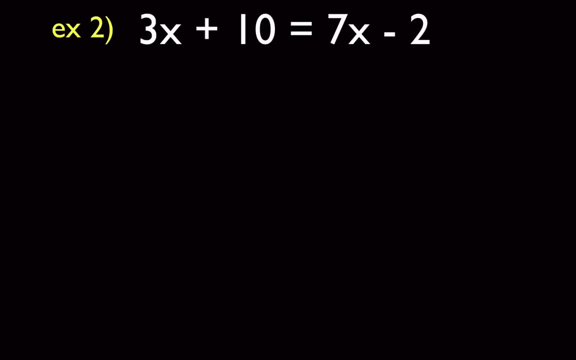 just to make sure, because I gave three different kind of variations, weird examples, to make sure you understand. So first thing we're going to do is we're going to get rid of the smaller of the two x's. So when I look at these two x's, 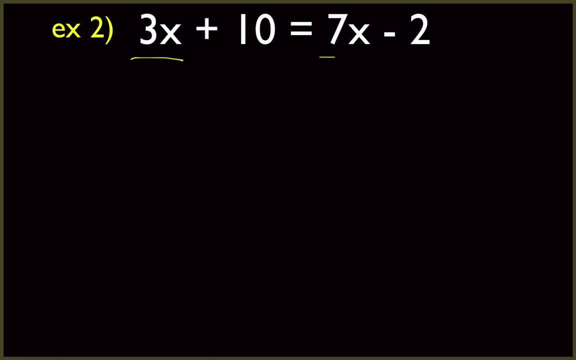 I'm talking about 3x and 7x. Which one of those is smaller? It would be 3.. So we're going to do the opposite of that, which is subtract 3. That's going to give me 4 on the right side and a minus 2.. 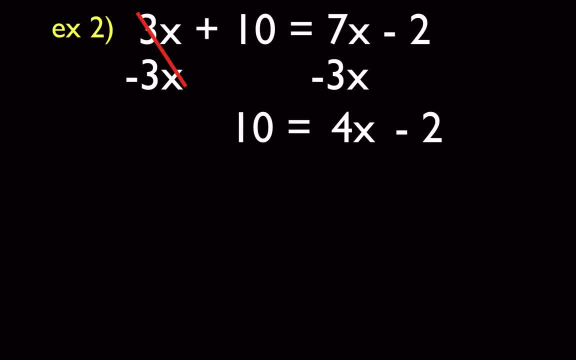 And on the left side, the x's are going to cancel, And all I'm going to be left with is 10.. Now from here, if you want to, you can then rearrange the problem to look like a common, comfortable, two-step equation. 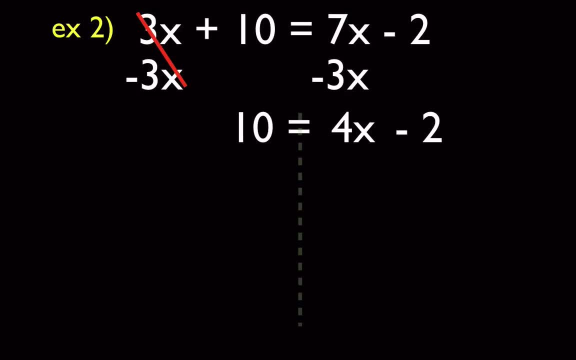 and then solve it from there, Or you can go ahead and solve it as is, Which means we're going to add 2 to both sides. On the right side it's going to cancel And we're going to end up with 12 equals 4x. 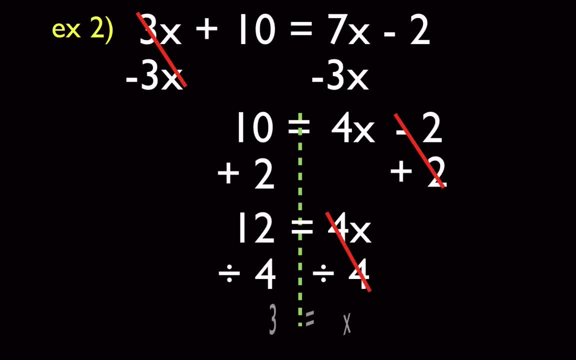 Dividing by 4, we'll get x equals 3.. It doesn't matter if it's 3 equals x or x equals 3. It's the same thing. But if that does give you a hard time or that bothers you, like I said, 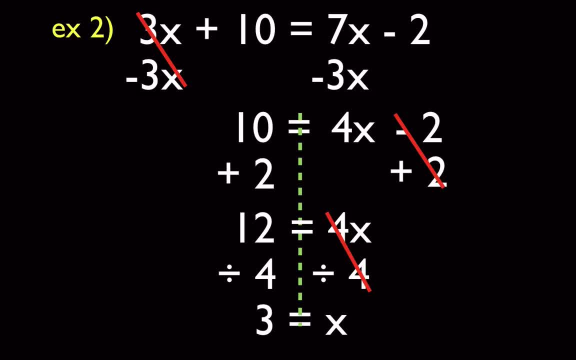 go back to that step and rearrange it when you have something like this happen. But, as you can see, we ended up not having to worry about negative x's. All we had to worry about was just the x's, Just the positive x divided by some number. 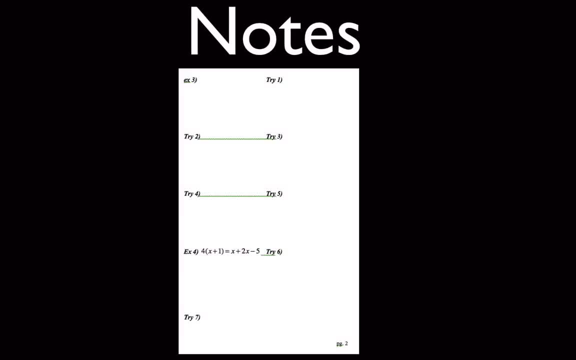 Okay, So now what we're going to need to do is we're going to need to move on to the second page of notes, which looks like this, So make sure you have that one in front of you. We're going to start on Example 3, on the paper in the top left. 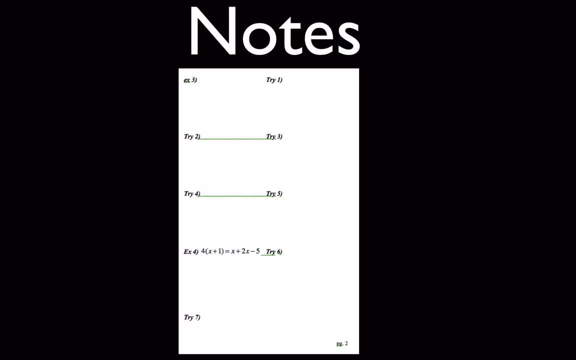 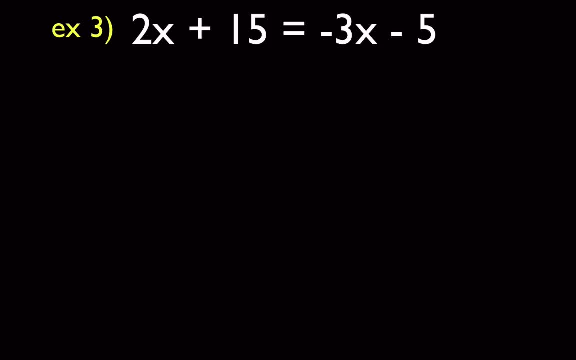 And then you can see you're going to do some practice problems together. Okay, So we're onto our last example now, before you guys try some on your own. So what I want you to pay attention to here is that thought of getting rid of the 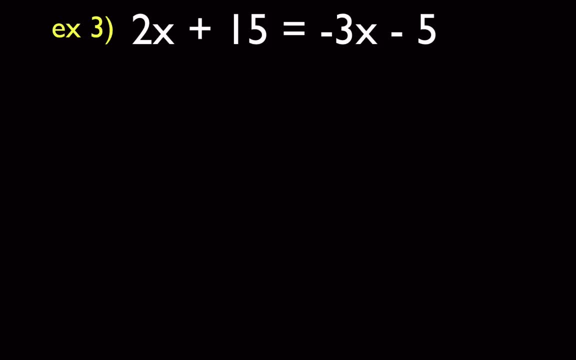 lower are the two x's. A lot of times people will want to go ahead and subtract two x from both sides because two is smaller than three, But two is not smaller than negative three. So remember, if you have one negative and one positive, you know the negative is always. 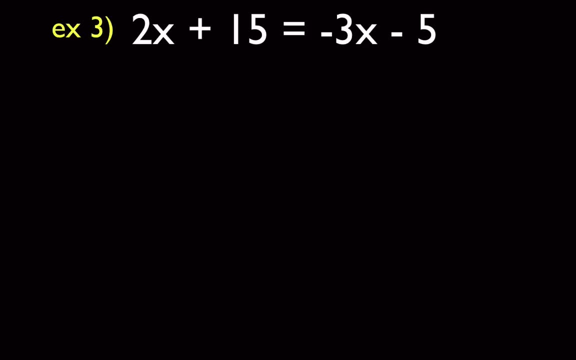 going to be what you're going to get rid of. If you have two negatives you want to get rid of, you know whichever one's more negative? Because more negative means well, I guess more negative is kind of silly. It's a lower negative, So something like negative ten versus. 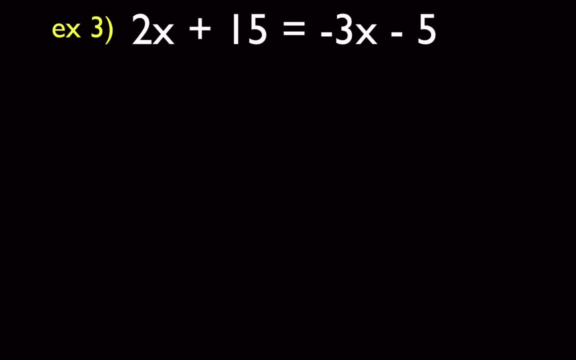 negative eight, you would get rid of the negative ten. So in this case we want to get rid of that three x. Notice that we added three x to both sides On all the other ones we subtracted. the reason is we want to cancel out the three x. So now I'm going to get five x fifteen. 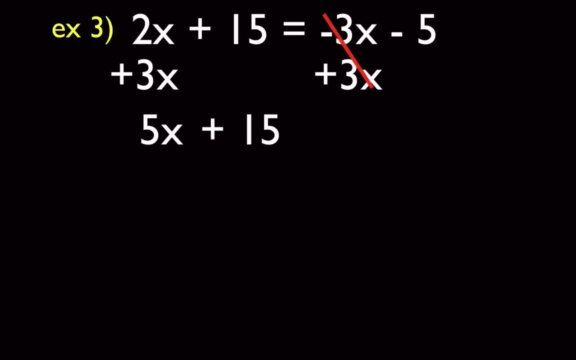 The x's are going to cancel. That's the point. you want that to be zero And negative. five comes down from above. Now we're at a two step equation. So we're going to follow our normal two step equation steps, Which is we're going to subtract fifteen from both sides And then divide by five. 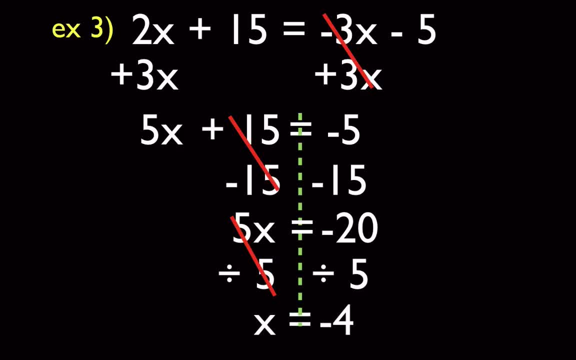 And we're going to get: x equals negative four. It didn't get rid of the possibility of negatives. We still have to deal with negatives. So be careful on this step, right here, Because that's where you might make a mistake to get that negative twenty. But at least we don't have 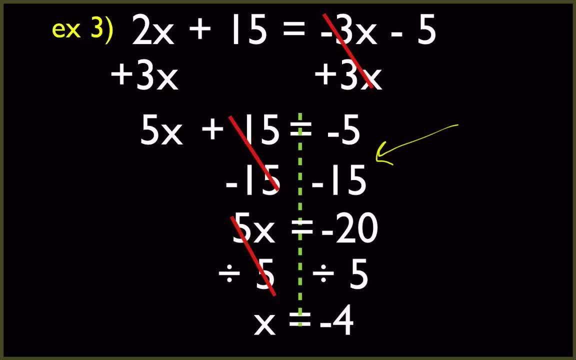 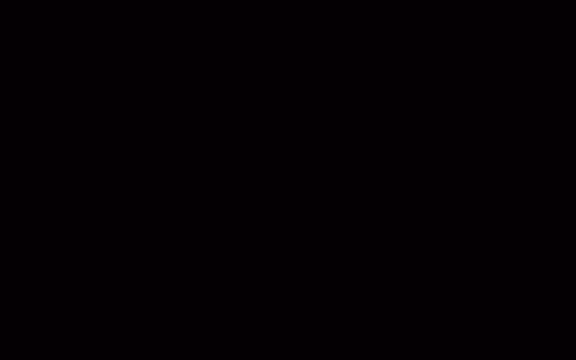 to divide by a negative, Because I know a lot of you guys get confused about, you know, dividing negatives. Okay, All right. So now what we're going to do is we're going to do an example on your own. So, as always, if you are unable to do it on your own, you can always pause the video. 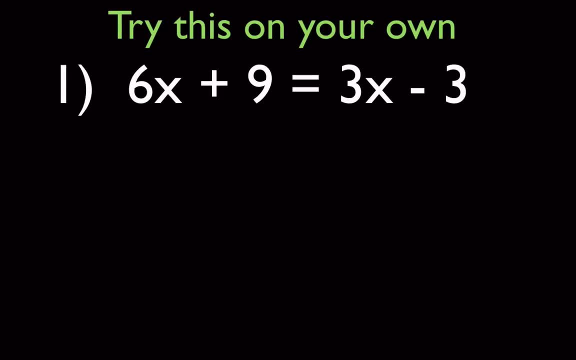 And then just give it a try And then try it again later. So this is number one. On the paper it says: try, Try one, try two, all the way up to five. Before you pause the video, though, I want to make sure you do not do one thing- A very, very common thing, people. 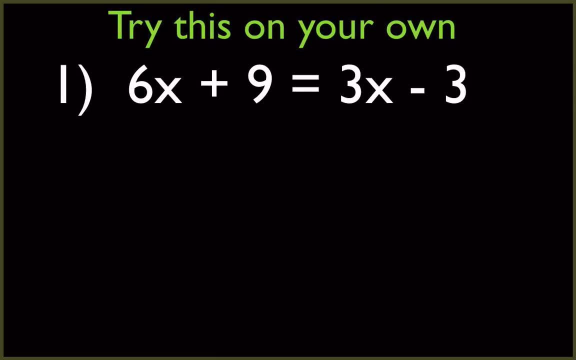 do is they try to do all of the steps at once. They say, oh okay, what I'm going to do is I'm going to go minus six x, And then I'm also going to go ahead and, do you know, minus. 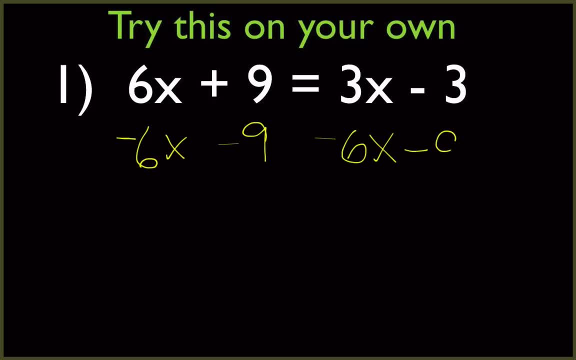 nine at the same time, And what they do is they're trying to get this thing done all at once. The problem is, what could happen is what I did here, Which is not only did I subtract the wrong one, but what I did is I subtracted everything from the left side. 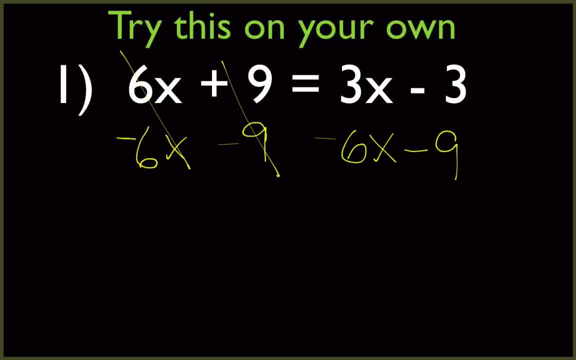 So this would cancel and this would cancel And I'd be left with zero. It's best to really just do one thing first. Give yourself a two-step equation and be comfortable with it. Don't try to do everything in one step. I will be marking those wrong, even if you get the right. 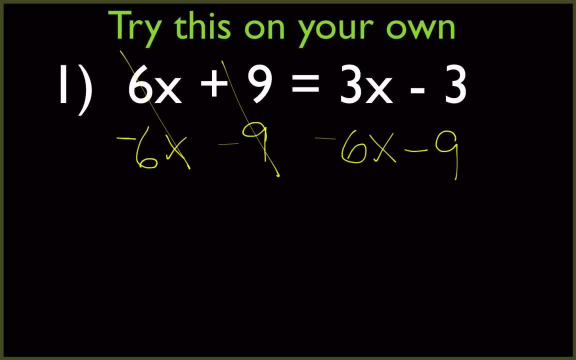 answer for doing that, Because it's a very, very common mistake students make. I understand some of you guys can do stuff in your head and everything, But there's a lot of people who do that And I'm going to show you how to do that And I'm going to show you how to. 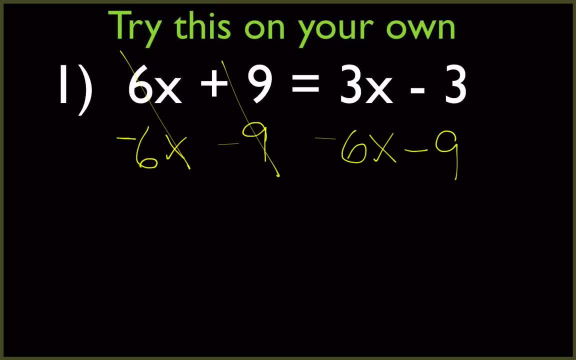 do that. There's a reason why we do three-step equations. with three steps. This is basically eliminating one of the steps, And everybody gets confused when it's equal to zero and they want me to tell them how to do it on a test And I can't do that. So build good. 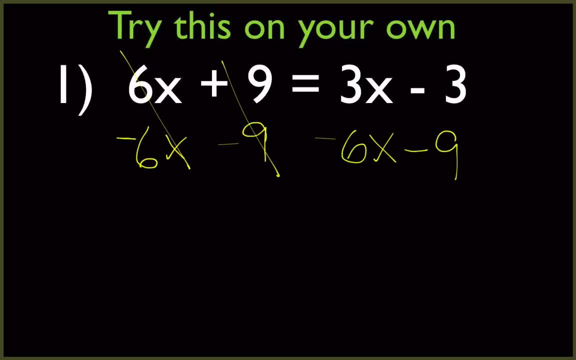 habits now. So go ahead, Give that a try. Pause the video, Hit play. after you got the answer, Go ahead and go over this problem. So the first thing I'm going to do is I'm going to subtract 3x, because 3 is less than 6.. That's going to leave me with 3x plus 9. 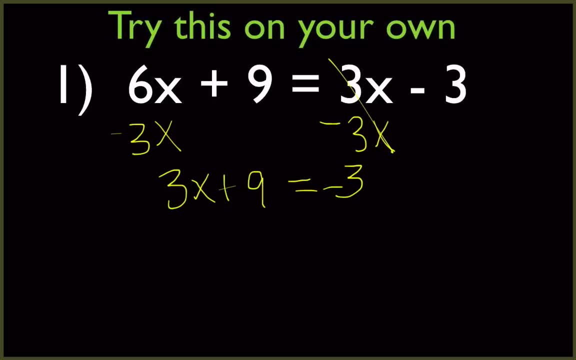 equals negative 3.. Okay, now I'm going to subtract 9 from both sides And I'm going to get 3x equals negative 12.. Dividing by 3 on both sides, I get x equals negative 4.. Okay, so, moving on to the next one, Still on that same page of notes, Go ahead and pause. 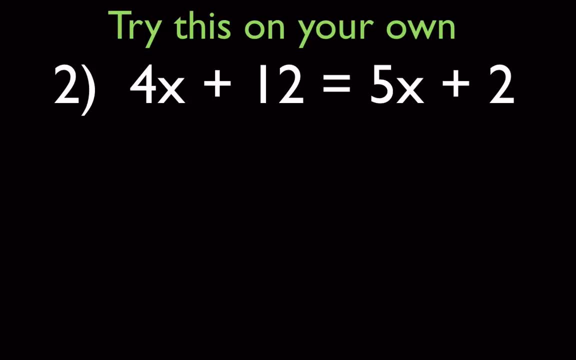 the video. Give this one a try on your own Hit play after you think you have your final answer. All right, so go ahead and get started here. First thing we're going to do is get rid of the lower of the x, which is 4x. That's going to cancel out And I'm going to be left. 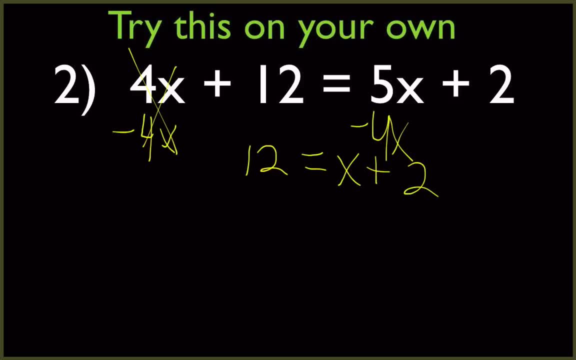 with 12 equals negative 4x. So I'm going to get rid of the lower of the x, which is 4x. 10 equals x plus 2.. 5 minus 4 is 1x, So I just wrote it as x. But if you put a 1 in, 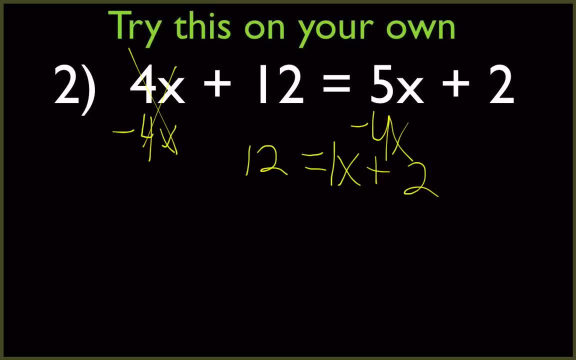 there, that's okay too. Now I need to go ahead and simplify: Subtracting 2 from both sides, I'm going to be left with 10 equals x, Just like before. remember, what we can do as well is we can easily check the answer. So 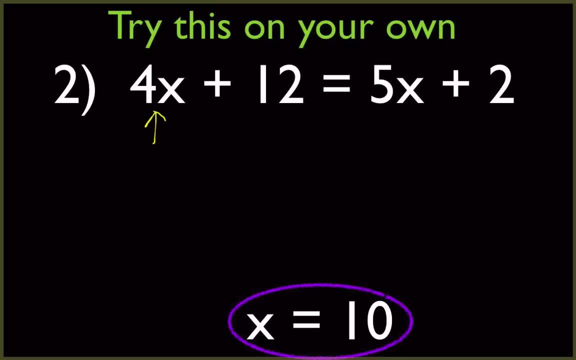 for example, if I take the lower of the x and I put it in the lower of the x, I'm going to take that 4 and I plug it in right here. I'm going to get 4 times 10 plus 12 equals. 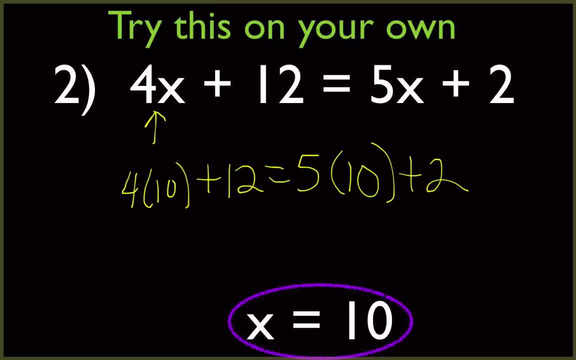 5 times 10 plus 2.. So I'm going to get 40 plus 12 equals 50 plus 2. And if you check those, both equal 52. so then we know we have the right answer. So again, remember that's. 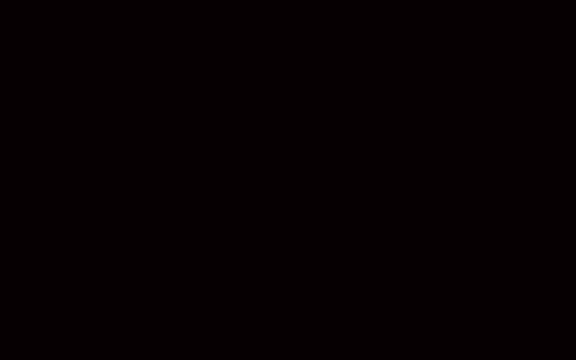 a great way to make sure your answers are correct. Okay, moving on to number 3, that you're going to try on your own, Go ahead and pause the video- Remember that that negative 2 is important on this problem- And hit play when you're done. 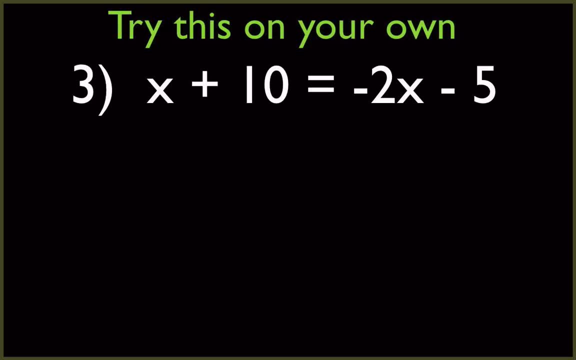 Alright, so go ahead and starting off here, First thing we have to do is get rid of the lower of the 2.. A lot of people might accidentally do minus x here. Remember you don't want to do that. I mean you can do that, but the easiest way to do the problem is going to be to go ahead and 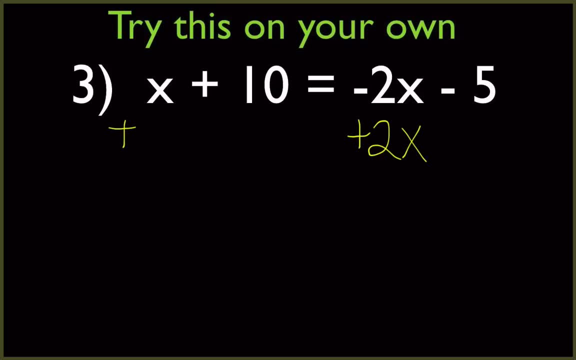 get rid of the lower, which is the negative. We're going to do opposite of it, which is adding. That's going to be gone And it's going to leave me with 3x plus 10 equals negative 5. Solving that problem from 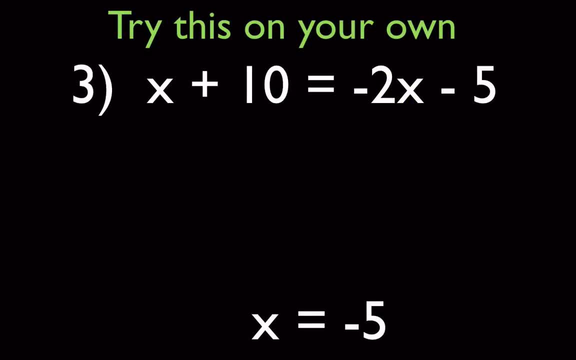 there, you're going to end up with negative 5 for your answer. And again, just raise your hand if you don't understand. you know the rest of the steps and I can come over, or Ms Allen can come over and help you out. Okay, moving on to number 4.. Both of these are negative. 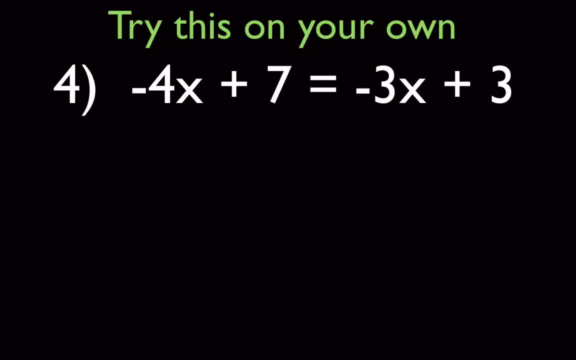 so be careful on which one you add Again. it will work out either way, But if you want the problem not to have negative, you have to be careful. So pause the video, give it a try, hit play when you're done. All right. So in this case, the best way to do it Is to get rid of the more negative number. 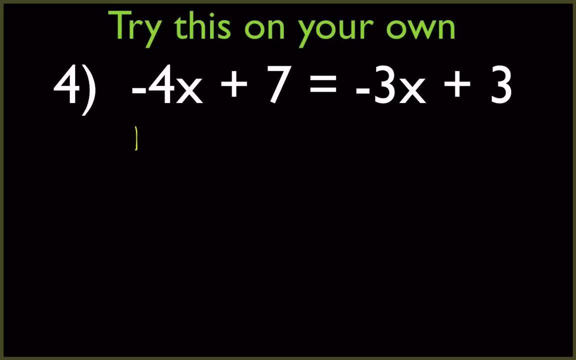 The number that is a further to the left on the number line, Which is actually negative 4.. So I'm going to add 4 x to both sides. That's going to cancel and I'm gonna be left with 7 equals x plus. 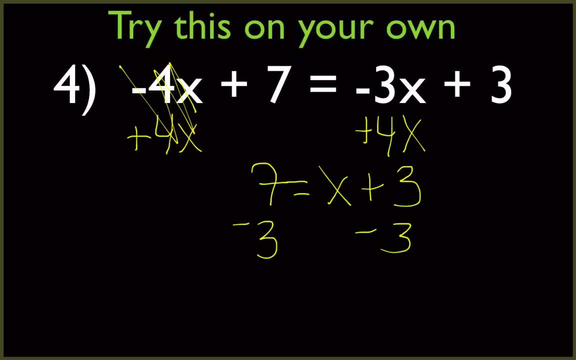 3.. It's actually just a one-step equation and I end up with x equals 4.. Again checking the answer, it'll end up being negative 16 plus 7,, which is negative 9.. And on the right side, negative 12 plus 3,, which is negative 9.. 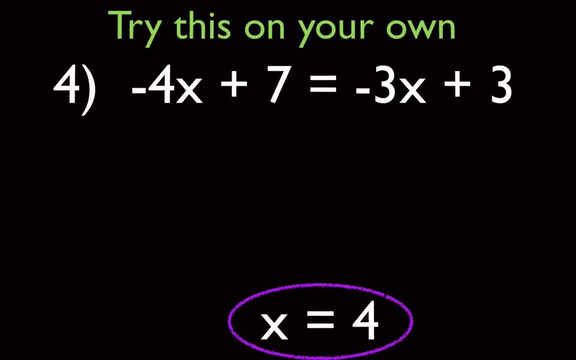 That just tells you, hey, I did it correctly. Okay, moving on to problem number 5.. The last one before we kind of put a spin on it. Go ahead and pause the video. give this one a try. hit play when you're done. 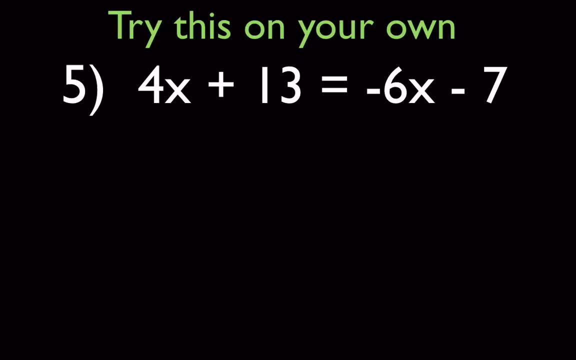 Alright. so what we're going to do is we're going to go ahead and get rid of the lower of the 2. Again, be careful here. that ends up being actually the negative 6. Which is going to give us 10x plus 13 equals negative 7.. 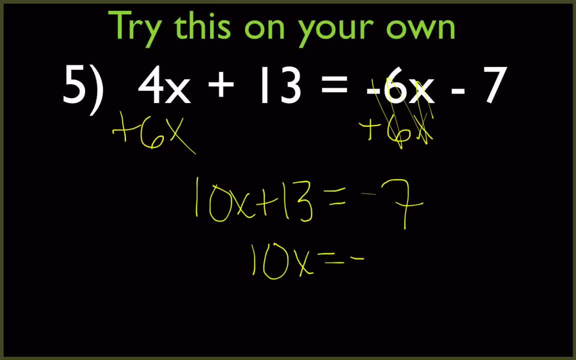 Subtracting 13 from both sides, you're going to get 10x equals negative 20.. This is a place where I want you to be careful. A lot of times people make mistakes on stuff like that, Especially when you're going negative. 7 minus 13 is negative 20.. 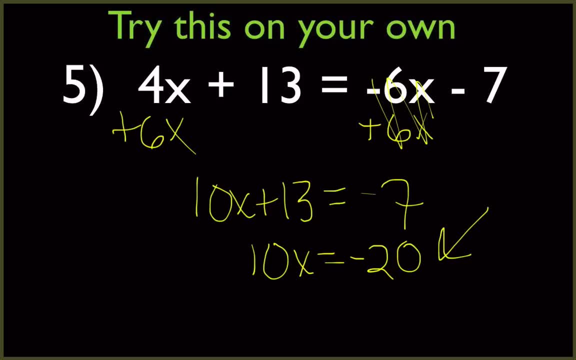 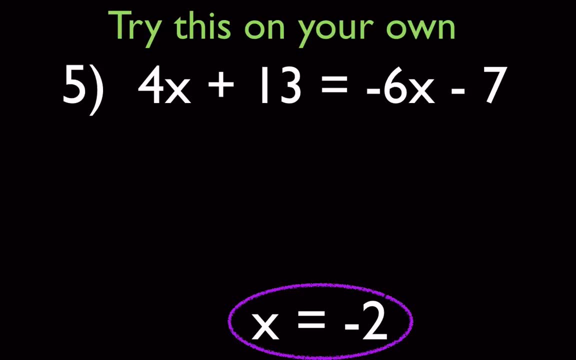 You owe $7, you borrow 13 more. now you owe 20.. Dividing by 10, you get x equals negative 2.. And again, very simple to check the problem, plugging it right back in. Okay, so still in the notes we're going to look at. 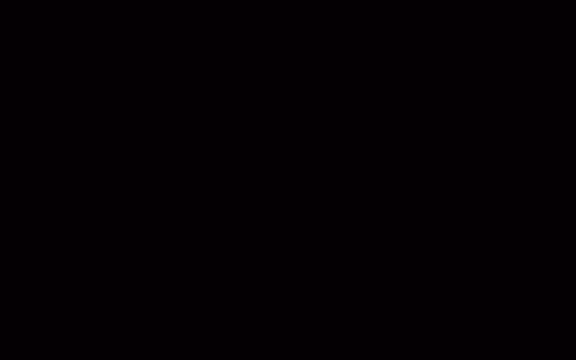 We're going to look at a fourth example, which is what if there's variables on both sides and it's sort of a you know multi-step on top of that? So, as you can see, on the left side we have what indicates a distributive property problem. 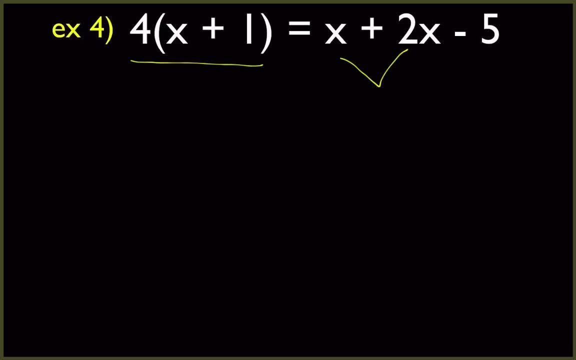 And on the right side we have what indicates a combining like terms problem. So what we're going to do is we're going to go ahead and first do the distributive property, And I got that 4x plus 4 by taking that and multiplying it by both. 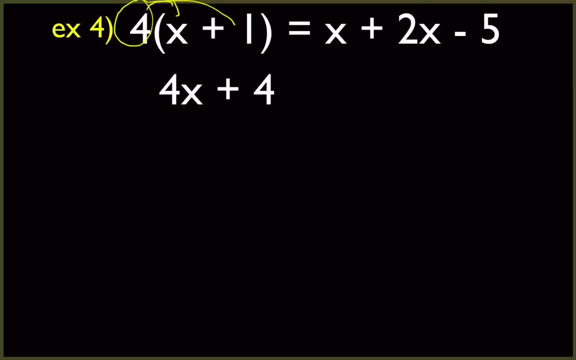 4 times x is 4x, 4 times 1 is 4.. On the right side, I'm going to combine like terms, Which is going to give me 3x minus 5.. So still applying what we learned earlier in the year. 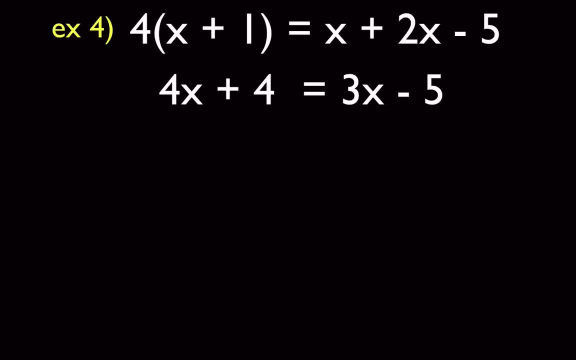 Now we have what amounts to an equation with variables on both sides. Be very, very careful not to combine like terms right here. That is again the most common mistake, And sometimes it still works out, and then you just will never know you had the wrong answer. 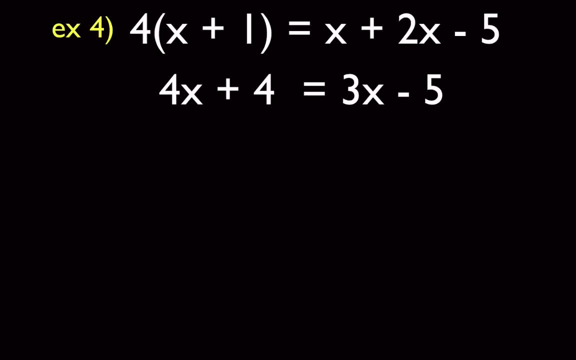 So now what we're going to do is we're going to go ahead and get rid of the lower of the two x's, which happens to be 3x. That's going to leave me with x, 3x plus 4, and, on the right side, negative 5.. 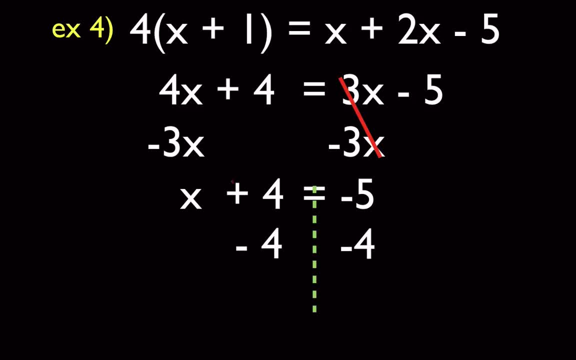 Subtracting 4 from both sides on our one-step equation, we get x equals negative 9.. So, as you can see, that's just a slight variation using the distributive property and combining like terms. So we're going to go ahead and do a couple more practice problems of those, to make sure you guys are comfortable. 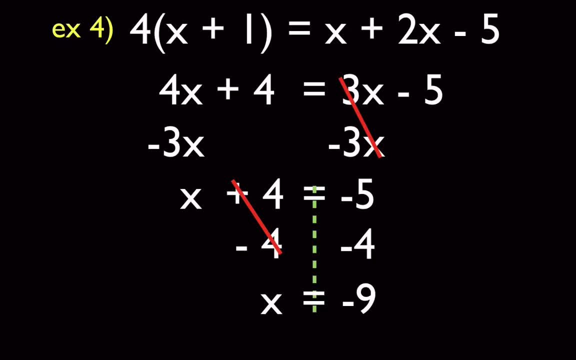 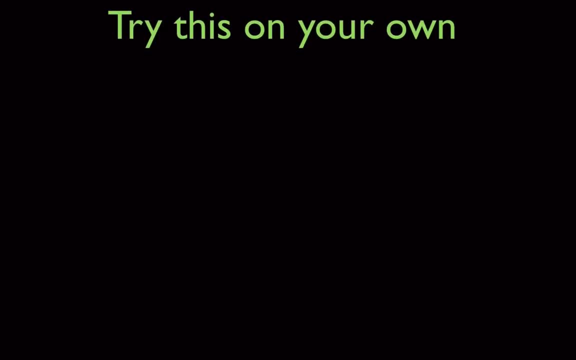 And then, after the video, there'll be an opportunity to do some extra practice. All right, so here's one to try on your own. As you can see, you have distributive property on both sides, so make sure you're careful about that. 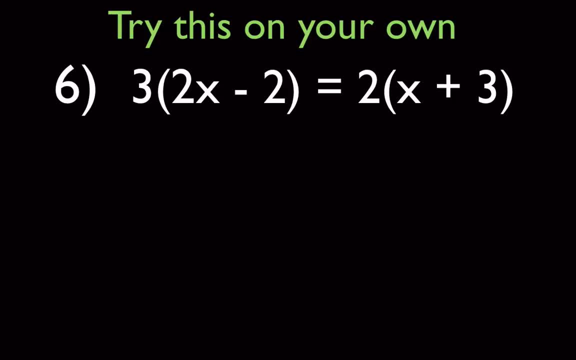 So pause the video, give it a try. If you're unable to get started, then let me do the first step before you pause it and then try to go from there. All right, so first thing we're going to do is we're going to distribute on both sides. 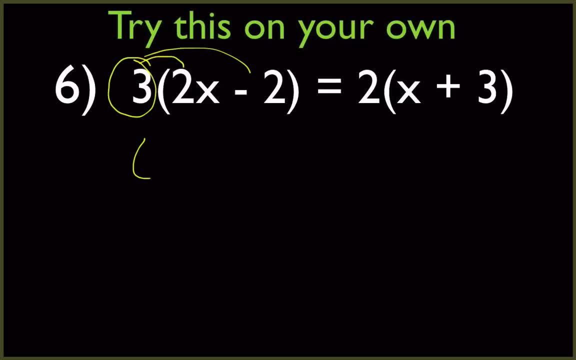 which is we're going to go ahead and take this 3 and multiply it And on the right side, we're going to take the 2 and multiply it. So, like I said, if you're unable to do the first step or you did it incorrectly, try pausing it right now. 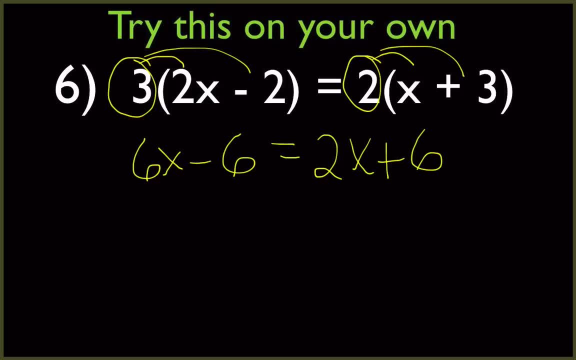 and just going ahead and you know, solve it from there and make sure you get that part of it, But you are responsible for knowing how to do even the more complicated versions. Okay, so now, from here, we're going to go ahead and get rid of the lower of the two x's, which is the 2.. 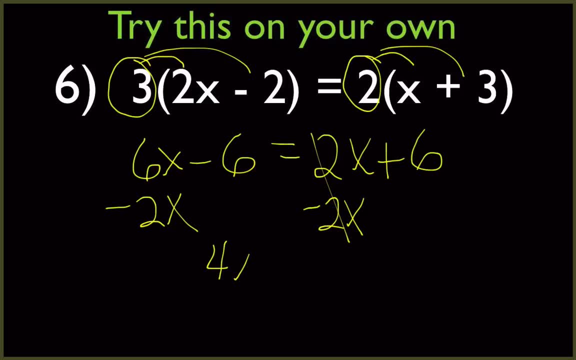 That's going to give me 4x minus 6 equals 6, which allows me then to go ahead and solve the two-step equation. Adding 6 to both sides, I'm going to get 4x equals 12.. So therefore, x equals 3.. 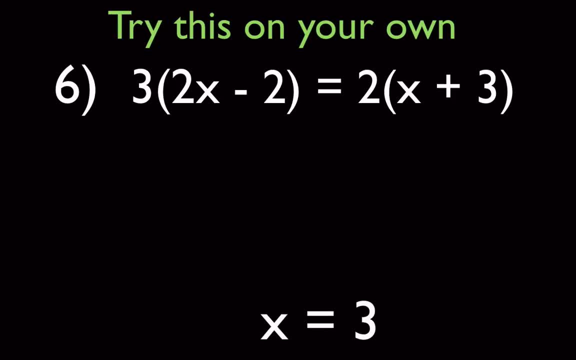 Okay, And I kind of ran out of room on the notes. So what I wanted you guys to do with that one is, you know, go ahead and solve it, but you can go to the right if you need to and make a second row. 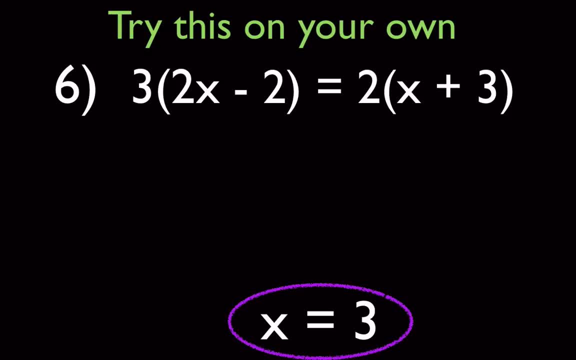 because I know there wasn't a ton of room in the notes. So, looking at number 7,, as you can see, here we end up with combining like terms on both sides. You could, of course, do problems that had combining like terms and distributive property. 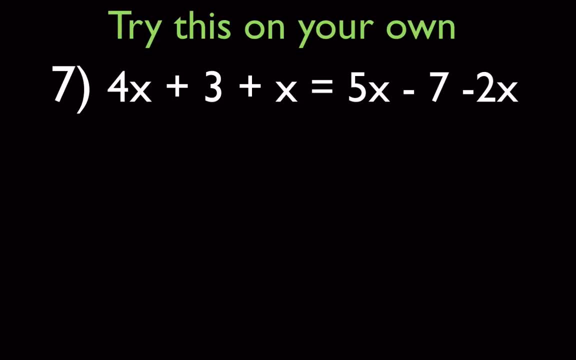 That'd be the most complicated version, but you guys did really well with that in class earlier this year, so I wouldn't worry too much about that. Just make sure that you follow the steps and do distributive property first. Okay, So pause this video. 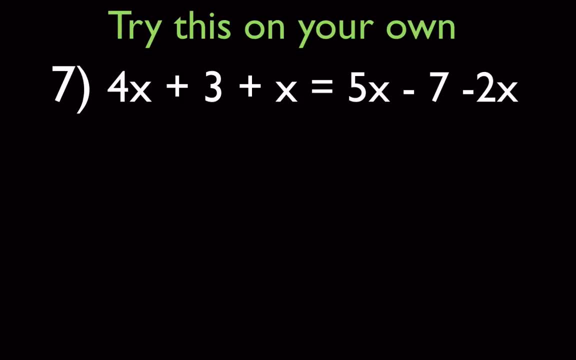 Remember you need to simplify both sides before you start moving x's. A lot of times I see people trying to do, you know, like minus x, plus 2x, minus 4x, and it's just very, very confusing when you do that. 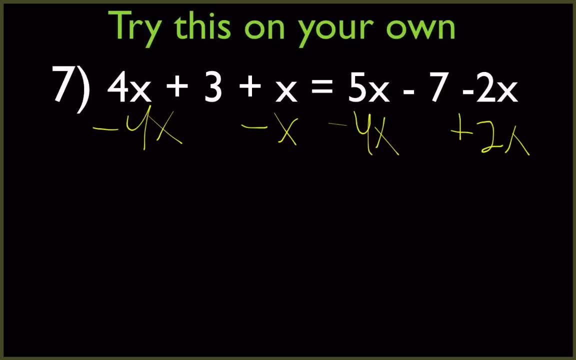 I mean, what's going on here? There's all kinds of stuff everywhere. How can you even balance that? You can't. You need to first get them neat. Then, when you get to a point where you have only one x on each side, 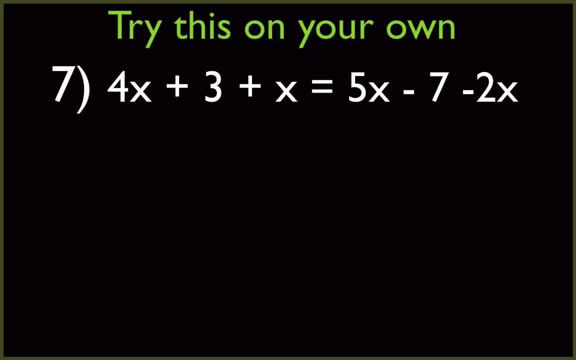 then you go through the steps to get rid of it. So pause the video, hit play after you're done or hit play after. Okay, Organize the first step. if you're unable to do that, All right. So, starting off here, I'm going to be combining my 4x and my x. 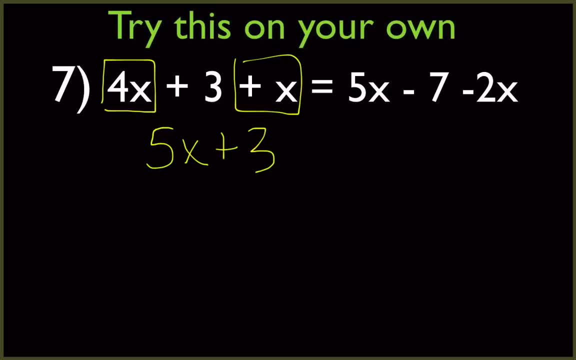 which is going to give me 5x and then my plus 3.. Notice, I'm only combining on one side of the equal sign. You cannot combine on both sides, only on one side. Okay, On the right side. now I'm going to combine my x's. 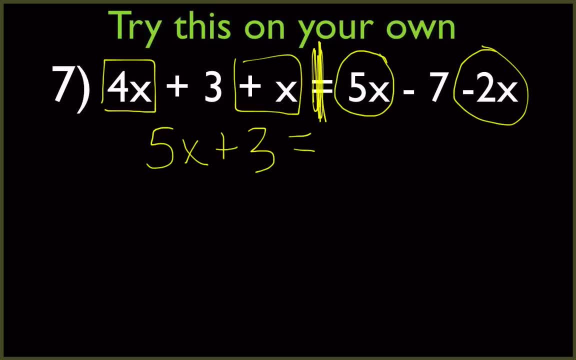 and I'm actually using a different shape so that I don't get confused. So now I've got 5x minus 2x, Which is 3x, And my minus 7 has nothing to combine. Now I'm at an equation with variables on both sides.